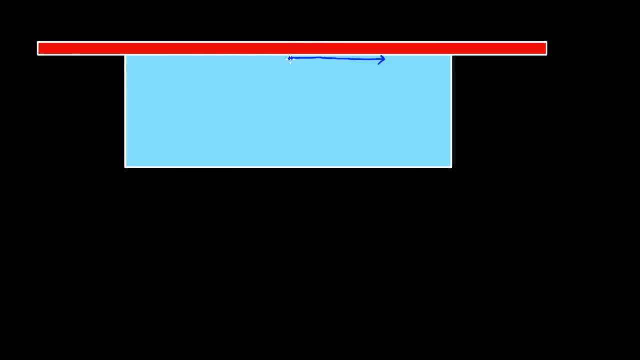 There's adhesive forces between this fluid and the lid On an atomic and molecular level. this fluid gets pulled with it. It resists the motion. but it's worse than that, because if this topmost layer gets pulled this way, then the layer right below it gets pulled by the topmost layer. This secondmost layer pulls this thirdmost layer. This keeps going down the line. What you get is a velocity gradient is the fancy name for it- which just means that this velocity of this fluid gets smaller and smaller Once you get down to the bottom. 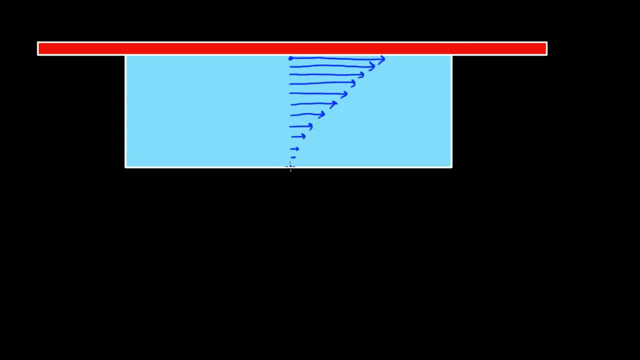 well, now the fluid is in contact with this surface at the bottom and this surface at the bottom is not moving. This fluid, that's at the lowest, most point, doesn't move at all. All right, so that's why this lid slowed down When we gave it a nudge. it was dragging that fluid along with it, and if it exerts a force to the right on the fluid, then the fluid is going to exert a force, by Newton's third law, to the left on the lid, and I'm going to call this a viscous force, I'm going to call it FV. 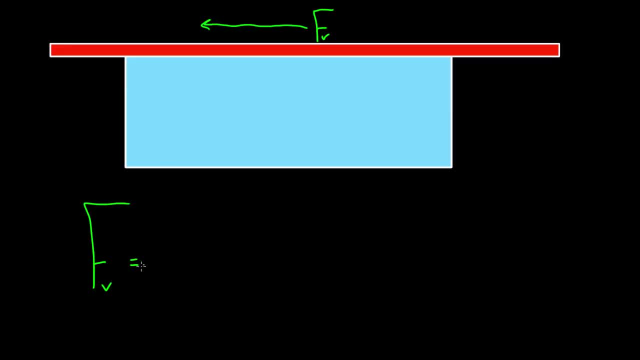 So what does this depend on? What does this viscous force depend on? One thing it depends on is the area, and not the whole area, of the lid. It's just the area of the lid that's actually in contact with the fluid. 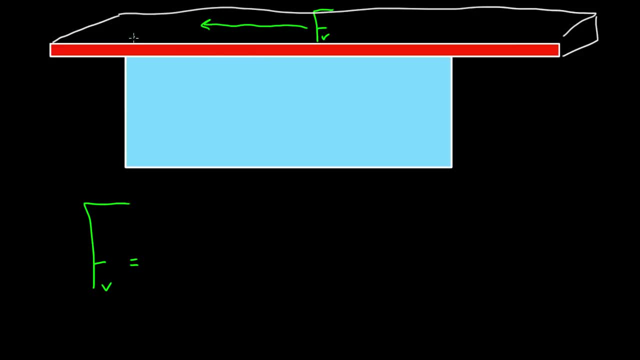 So, if you imagine, the dimensions of this box would only expand here. so it's only that part of the lid that's actually in contact with the fluid. So that area and it's proportional to that area. The bigger that area, the more fluid you're going to be dragging. 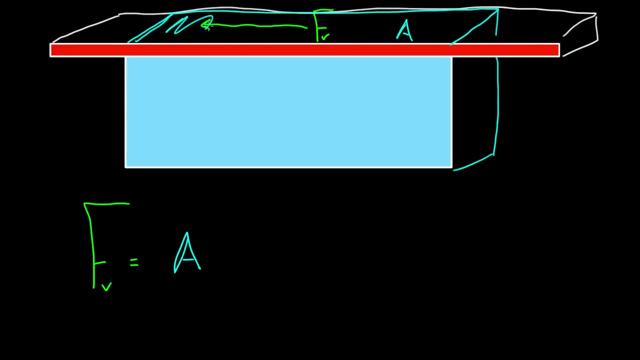 the larger the viscous force That makes sense. so it's this area here, And something else that it depends on is the speed with which you drag the lid. So the faster I pull the lid, well, the faster I'm going to be pulling this water. 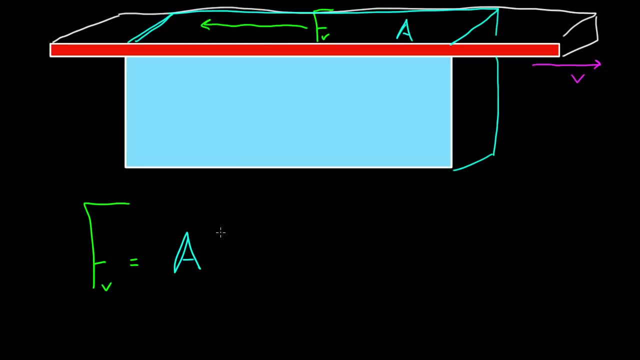 the bigger that force, which means the bigger the viscous force. so it's proportional to the speed as well. It's inversely proportional to the depth of the fluid. I'll call that D. And then it depends on one more thing: It depends on the 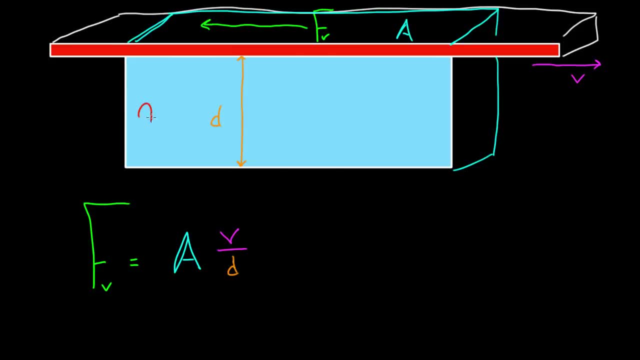 viscosity of the fluid, Maybe the most important factor in this whole discussion. eta is going to be called the viscosity of the fluid or the coefficient of viscosity, And what this number tells you is how viscous, how thick, essentially, the fluid is. 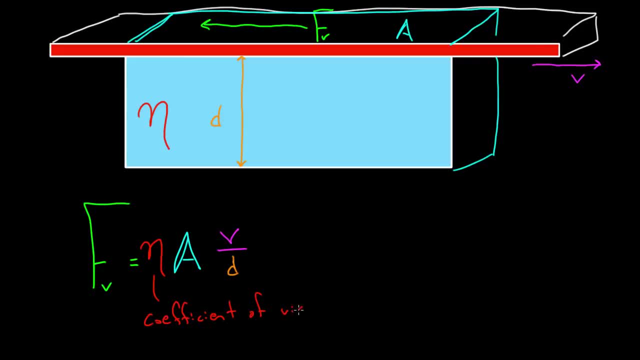 How much it resists flow And so coefficient of viscosity. so, to give you an idea, honey or corn syrup would have a large viscosity, Water would have a smaller viscosity coefficient And gases would have a coefficient of viscosity even less. So what are the units of this? 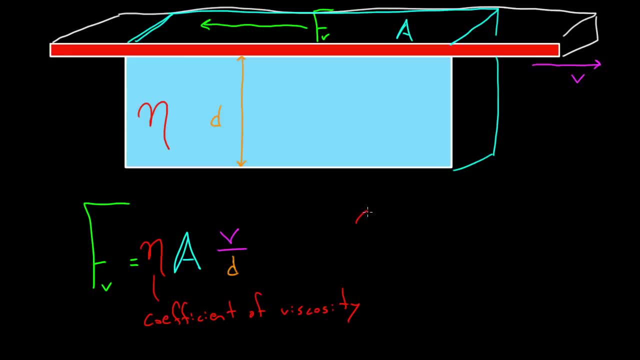 coefficient of viscosity. Well, if we solved, if we were to solve for the eta, what would we get? We'd get force divided by area. so this would be force divided by area and multiplied by the distance, divided by the speed. What units do these have? Force is in. 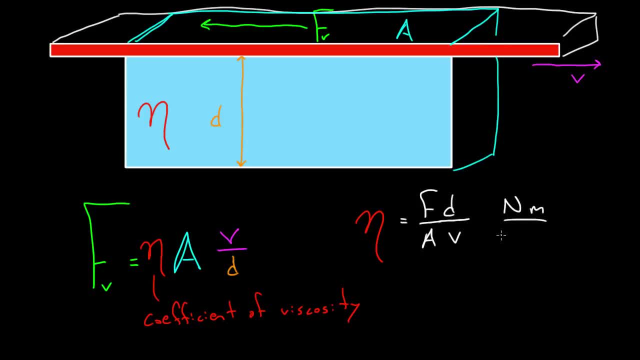 newtons. Distance is in meters, Area is in meters squared Speed is in meters per second. So I bring that second up top, because it was divided in the denominator. So it goes up top. And what am I left with? Meters, cancels, meters. 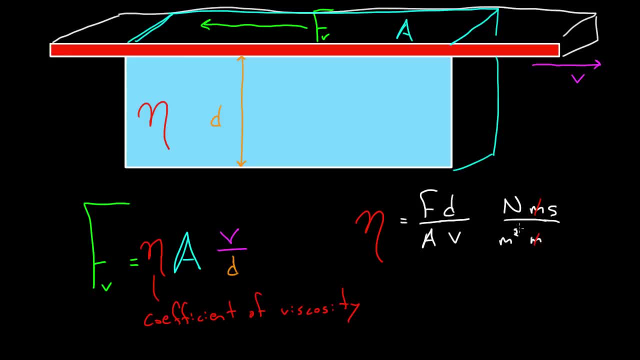 And I'm left with the units of viscosity as being newtons per meter squared, times a second. But a newton per meter squared is a pascal, So this is pascal seconds. So these units are a little strange. but the units of eta. 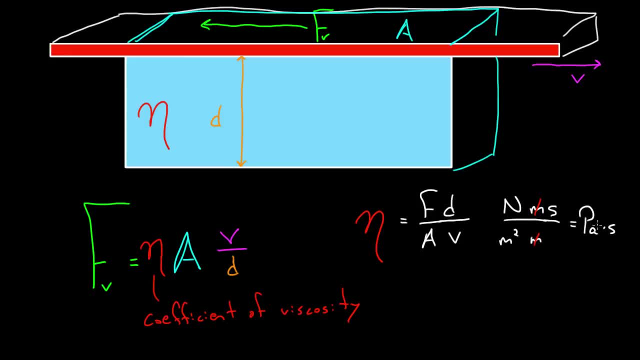 the coefficient of viscosity is a pressure times a second, Pascal seconds, But some people use the unit poise, and one poise is equal to one tenth of a pascal second, Or in other words ten poise, and it's abbreviated capital, P. 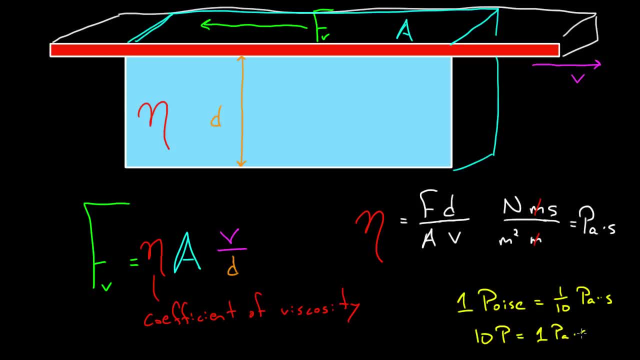 is one pascal second, And so you'll often hear this unit poise as a measure of viscosity. So what are some real life values for the viscosity? Well, the viscosity of water at zero degrees Celsius is- and I'm not talking about ice, but water. 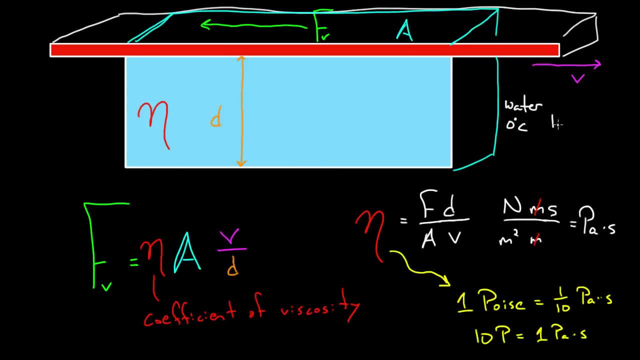 that's actually at zero degrees but not frozen yet, is about 1.8, but 1.8 milli pascal seconds. And another way to say that: look at milli pascal seconds. that would be a centa, a centa poise. 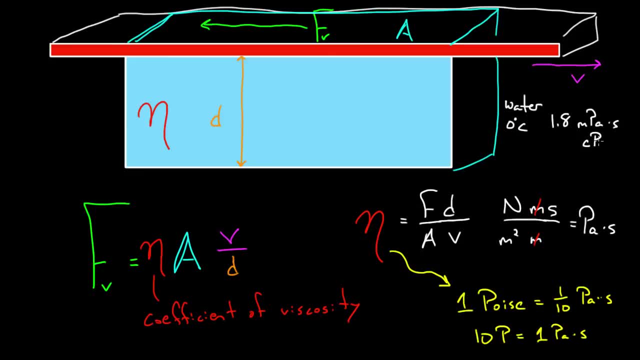 CP, Because a poise is already one tenth of a pascal second. Remember, one poise is one tenth And so a centi poise is really a milli pascal second. Or water at 20 degrees Celsius is: 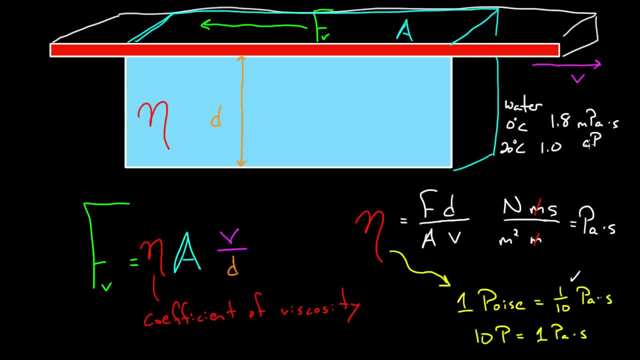 1.0 milli pascal seconds or centa poise. Now you can see there's a huge dependency on temperature. The viscosity is highly dependent on temperature. The colder it gets, the more viscous a fluid typically gets. 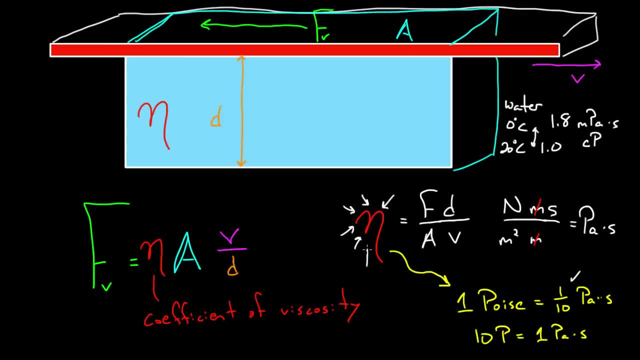 Which you know, because if you start your car and it's too cold outside, that car's not going to want to start, That oil inside is going to be more viscous than it's prepared for and that engine might not start very easily. 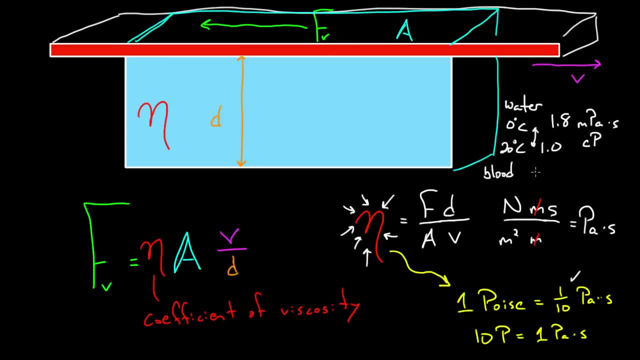 Blood typically has a viscosity between 3 to 4 milli pascal seconds, or centa poise. And then engine oil can have viscosities in the hundreds around 200 centa poise. And then gases. gases would have viscosities that are even less. 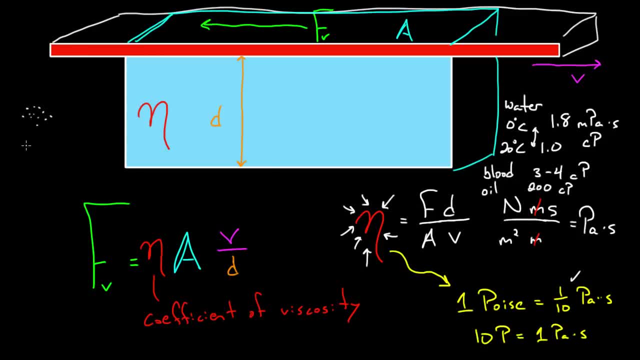 Air has a viscosity of around 0.018 centa poise. Now it's important to note if a fluid follows this rule, for the viscous force and the coefficient of viscosity does not depend on the speed with which this fluid is flowing or with which you pull. 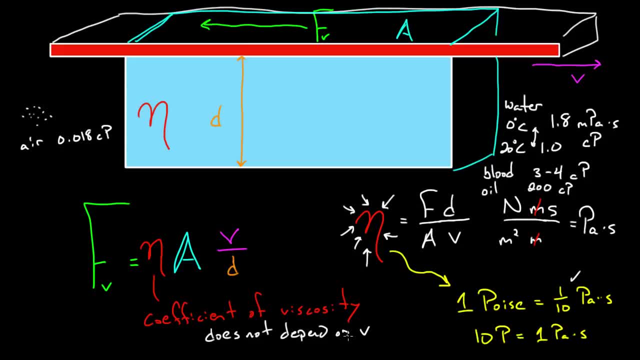 this lid over the top does not depend on that, then we call this a Newtonian fluid. Then it's a Newtonian fluid. But if the coefficient of viscosity does depend on the speed with which the fluid is flowing or the speed with which you pull this lid, 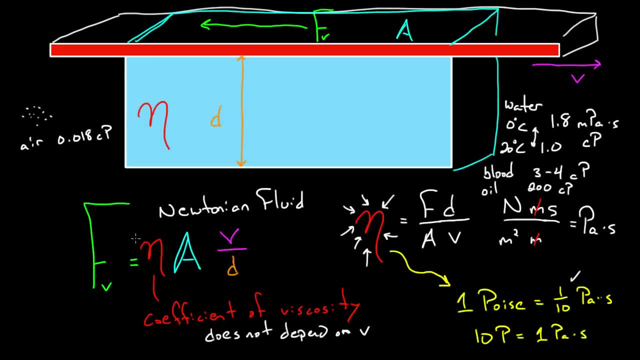 then it would be a non-Newtonian fluid. So if this coefficient of viscosity stays the same, regardless of what the speed is, it's a Newtonian fluid. If that's not the case, it'd be a non-Newtonian fluid. Now. 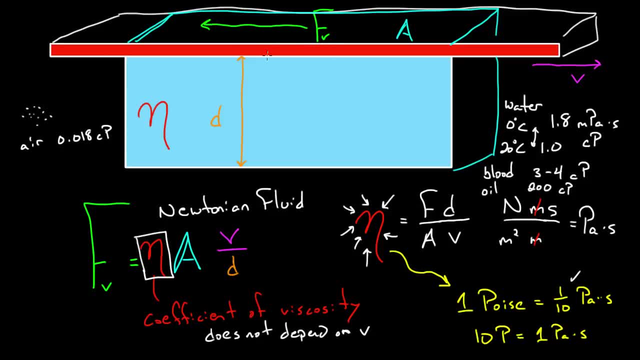 you might be thinking: well, this is kind of stupid. I mean, how many cases are we going to have where you're trying to pull a lid over a box? You've probably never tried to do that in real life, But this is just a handy. 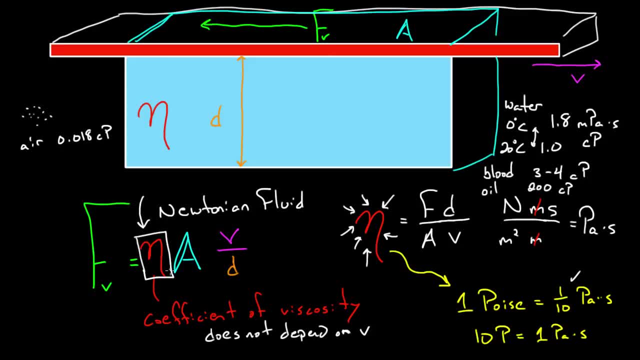 way to determine the viscosity. Once you know the viscosity, you can apply this number. This is a constant of the fluid. Now, anywhere that this fluid is flowing, now that you've measured it carefully, you can determine what kind of flow rate you would get. So imagine: 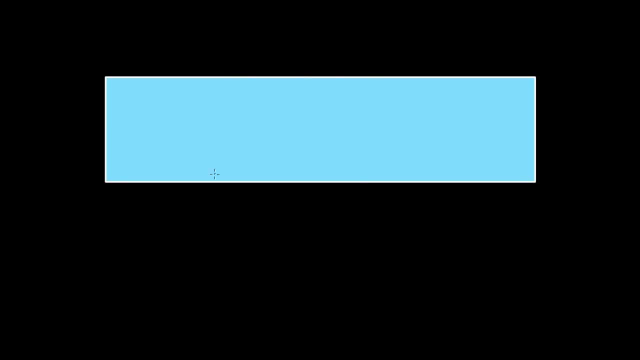 let's get rid of all this stuff here. say, you had a stationary tube or a pipe and there was a fluid flowing through it. Maybe it's a vein or a vessel and it's blood flowing through it. Anyways, now it's stationary though. 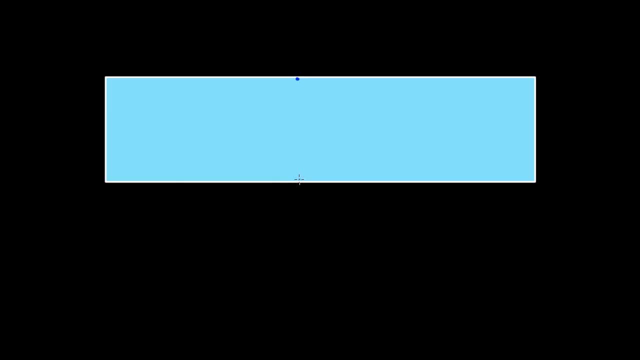 Both the top and the bottom are stationary, so that means the fluid near the top and the fluid near the bottom aren't really moving, but it's the fluid in the middle that's moving fastest and then slightly less fast, and you get this. 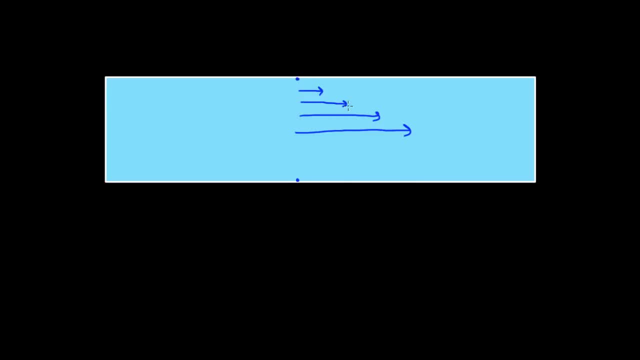 somewhat parabolic type velocity gradient, where it gets bigger and bigger and then it gets smaller and smaller, and so the velocity profile might look something like this: and if we wanted to know how much volume of fluid, how many meters cubed of fluid pass by a certain point. 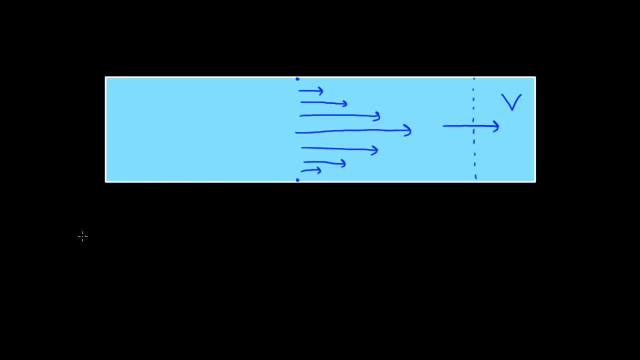 per time. we can figure that out. There's a formula for this: The volume per time, the meters cubed per time. the formula's called Poiseuille's Law and it says this: It says the volume that will flow per time. 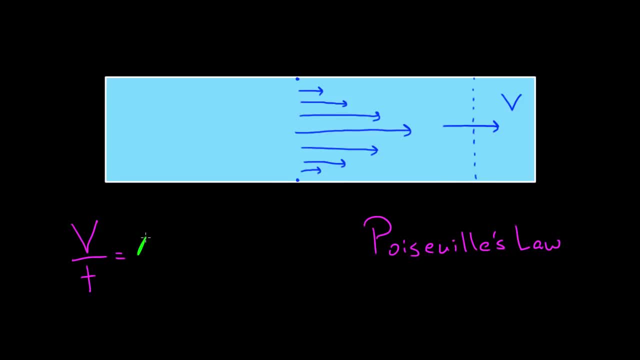 is dependent on delta, p times, pi times r to the fourth, divided by eight eta times l. Now, this is a crazy equation. Let's break this thing down and see what it's really talking about. So here's Poiseuille's Law. So 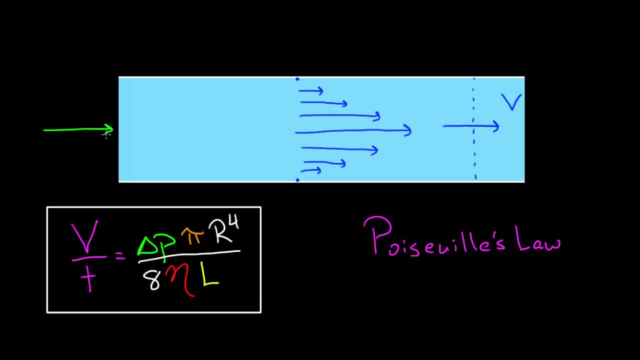 this delta p is referring to the pressure differential. so there'll be pressure on this side. We'll call it p1.. There'll be pressure on this side- P2,. if those are the same, this fluid's not going to be flowing very long. There has to be a difference. 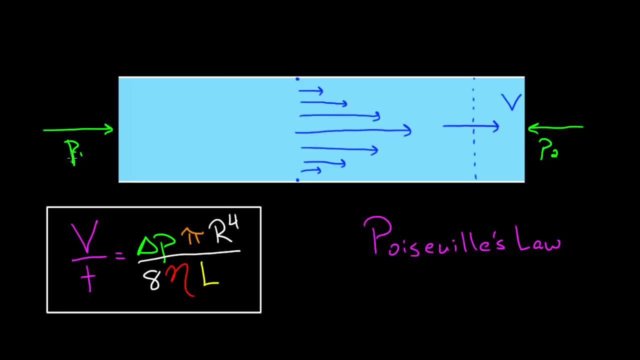 If we want the fluid to flow to the right, p1 has to be bigger than p2, and the greater the difference. the greater this difference, p1 minus p2,, the more volume that's going to flow per time and that.